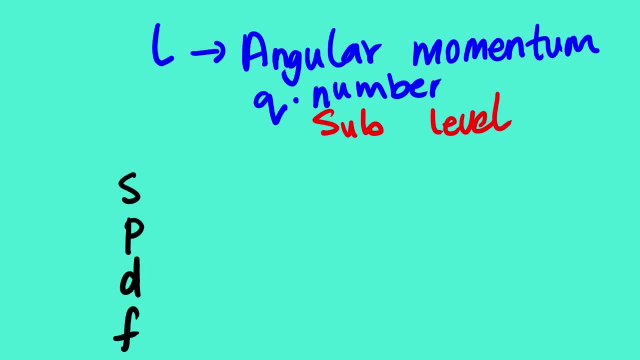 It describes the sub-levels. Remember, we talked about the energy levels, or the levels, which is the value of N. For the sub-levels, we are using angular momentum quantum number, which is letter N. This is what you must know. 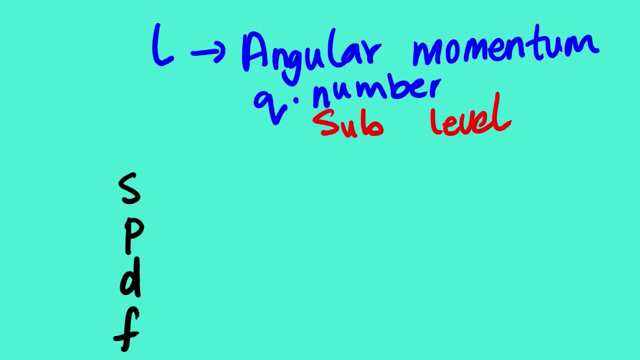 As you all know from the previous lesson videos, we have s, p, d And f orbitals, All the s orbitals. the value of their angular momentum is zero, So it doesn't matter whether we have 3s, 4s, 1s. 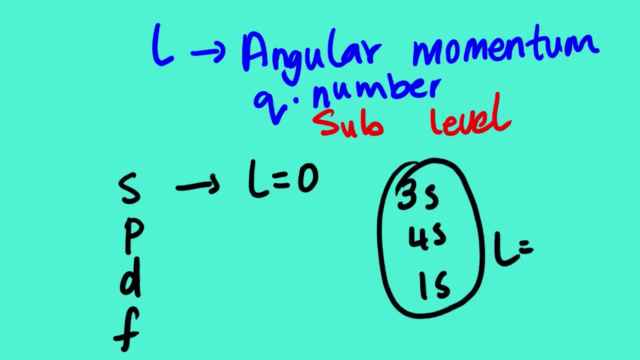 Just know that the value of this orbitals is- I mean the value of the angular momentum for this orbitals- is zero. You should take notes. We are going to use this information When answering the questions. Now for p orbitals. all the p orbitals. their angular momentum is equal to 1.. 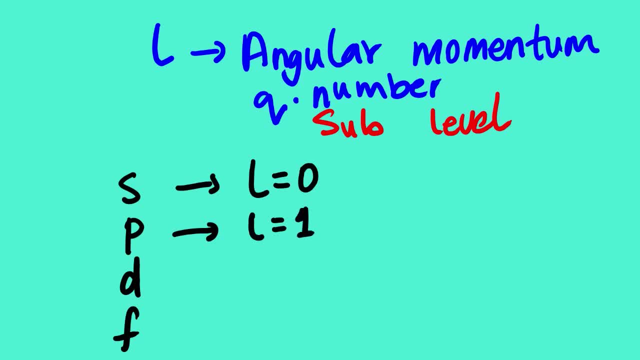 d orbitals: all the angular momentum is equal to 2.. f orbitals: all the angular momentum is equal to 3.. We are going to use this. Just know that s is equal to zero, p is equal to 1.. 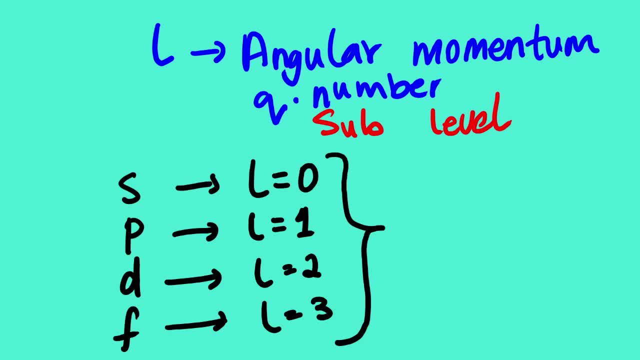 d is equal to 2.. f is equal to 3.. That is the sub-levels. It describes the sub-levels of energy levels. Let us look at the relationship between the energy levels and the sub-levels: The principal quantum number and the angular momentum quantum number. 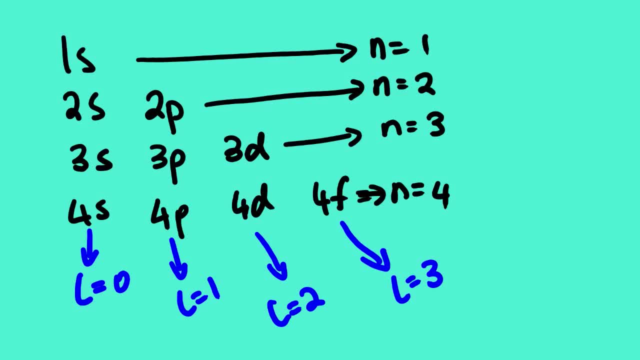 This diagram illustrates what we've talked about so far. from the beginning of this lesson video, We said: the s orbital, the sub-level is zero. And then, for the p orbital, the sub-level is 1.. For the d orbital, the sub-level is 2.. 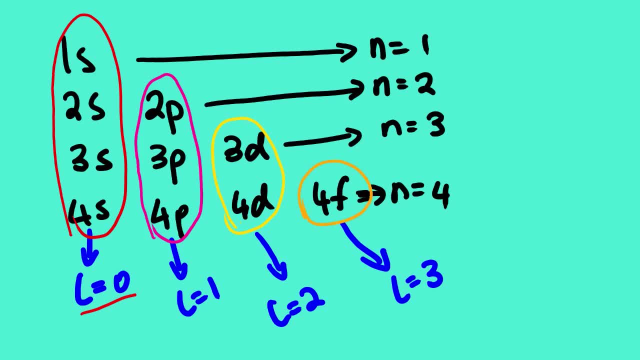 The f orbital, the sub-level is 3.. And then we also said: under 1s the energy level is: n is equal to number 1.. That is the principal quantum number For energy level. number 2, n is equal to 2.. 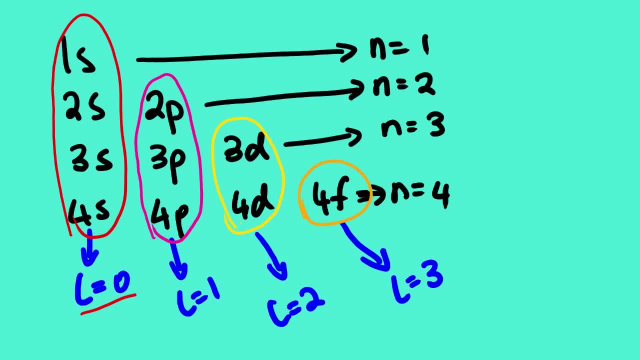 We have two orbitals, which is s and p. n is equal to 3.. We have three orbitals which is s, p, d And then energy level, number 4, we have four orbitals which is s, p, d, f. 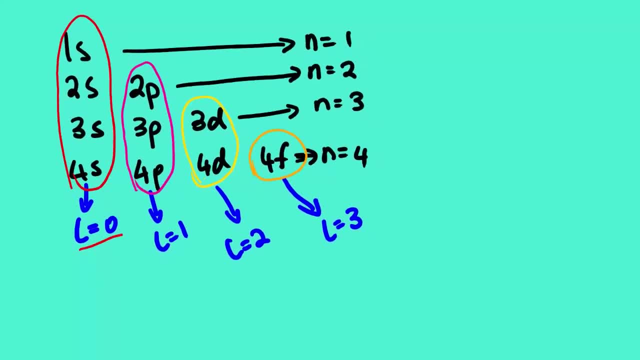 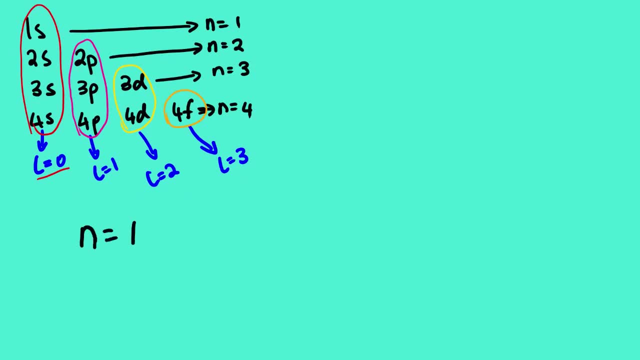 Now we need to look at the relationship between the two. Under energy level, number 1, n is equal to 1.. Let me actually write it here: n is equal to 1.. You can see that we only have one orbital, So we said s orbital. 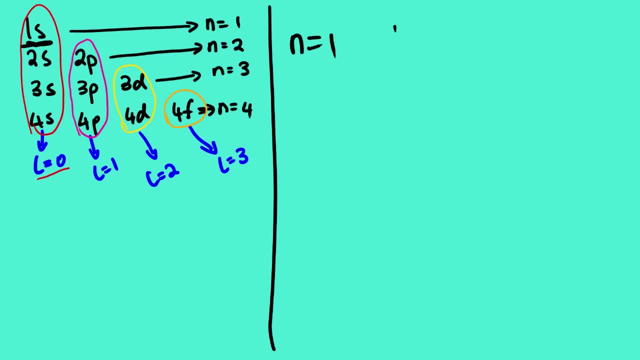 the angular momentum for s orbital is. let me write it like this: We only have one, s, And then the angular momentum is: l is equal to zero. Looking at energy level number 2, we have two orbitals, which is s and 2p. 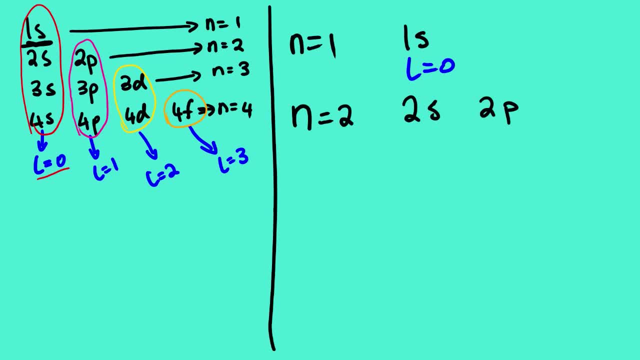 Now we said: for the s orbital the angular momentum is 0.. For p orbital the angular momentum is 1.. So for second energy level, n is equal to 2.. We have two angular momentum which is l is equal to 0 for s orbital. 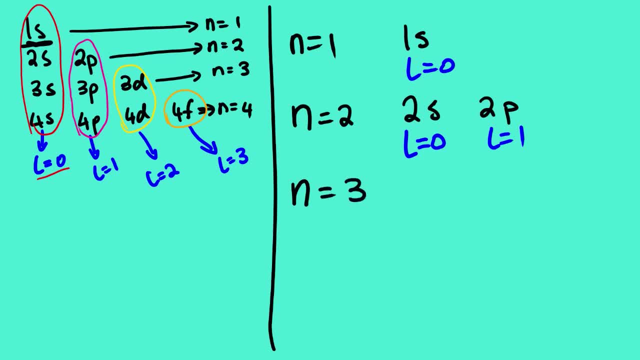 l is equal to 1 for p orbital, And then energy level number 3, we can see that under 3, we have three orbitals: It's 3s, 3p, 3d, So it means our angular momentum. 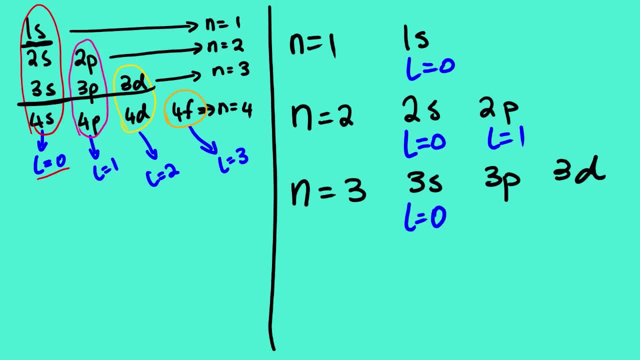 quantum number will be 0.. Or the sub energy level will be: l is equal to 0, l is equal to 1, l is equal to 2.. So under 3 energy level we have three angular momentum. We continue. 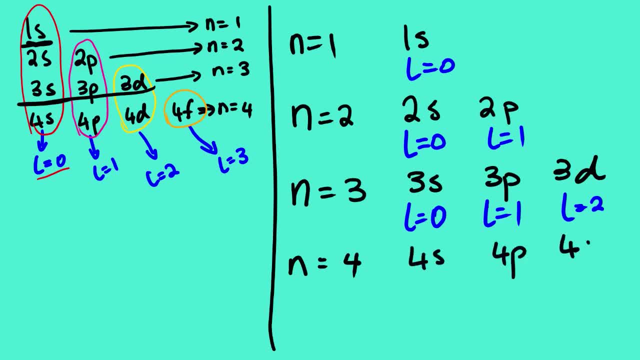 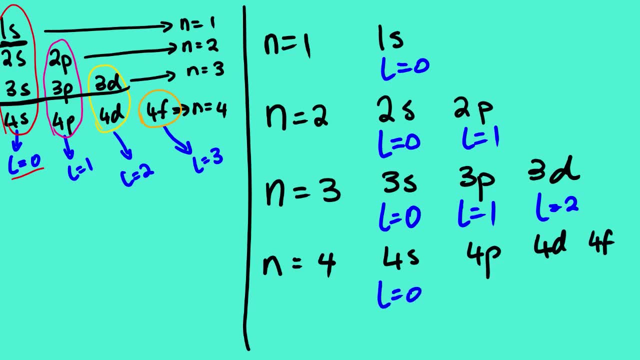 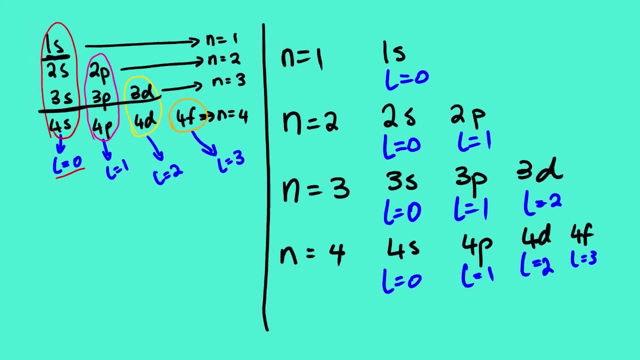 We have 4s for p, for d and for f, So you can see that we have: l is equal to 0, l is equal to 1, l is equal to 2, l is equal to 3.. Master this. 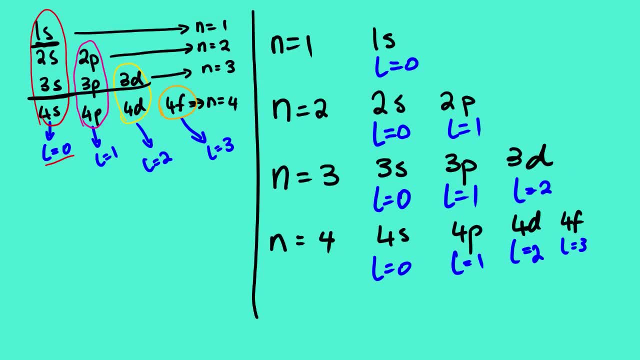 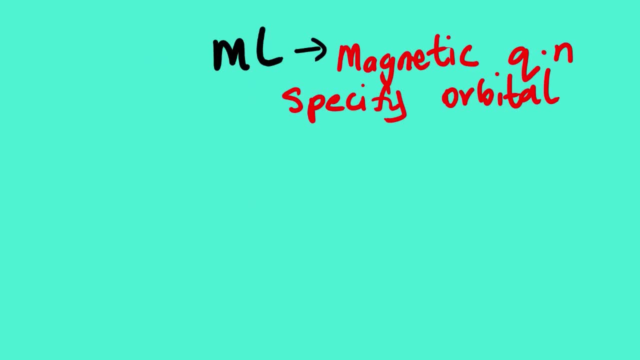 We are going to use this. Let us continue. ML is one of the quantum numbers, which is the magnetic quantum number. It specifies the orbital or it specifies the electron in an orbital. Let us try to explain this If you still remember the orbital diagram. 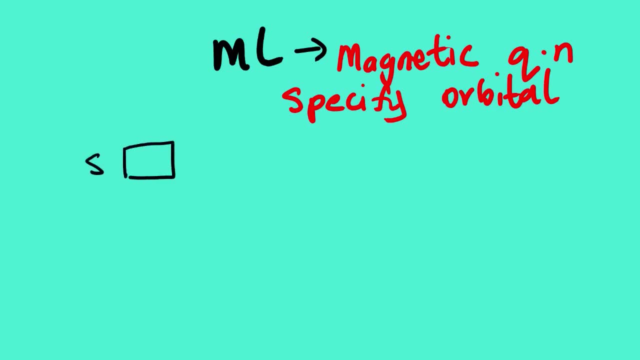 we said the s orbital has only one box, The p orbital has three boxes, The d orbital has five boxes, Then the f orbital will have seven boxes. Now we should know this. When we bring the knowledge of our sub-levels, we actually know that for s orbital. 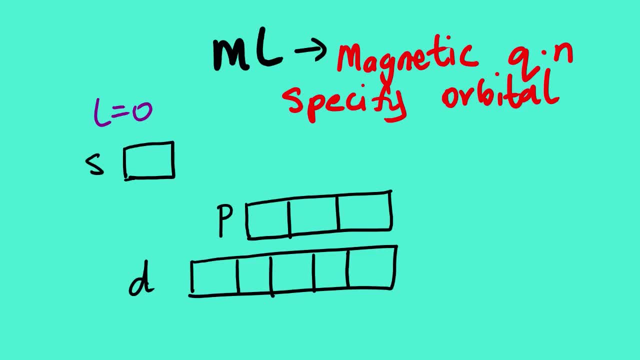 l is equal to 0. And then this simply means that for our magnetic quantum number, ML, we are going to have 0.. Let us go to the p orbital. We know that the sub-level of p orbital l is equal to 1. 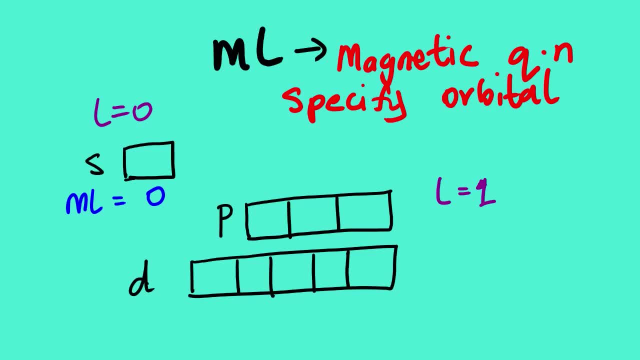 for p orbitals. This simply means that for ML, just know that if our sub-level is 1, then it means our ML will start from negative 1, 0, 1.. I hope you can see the trend Now. we know that the d 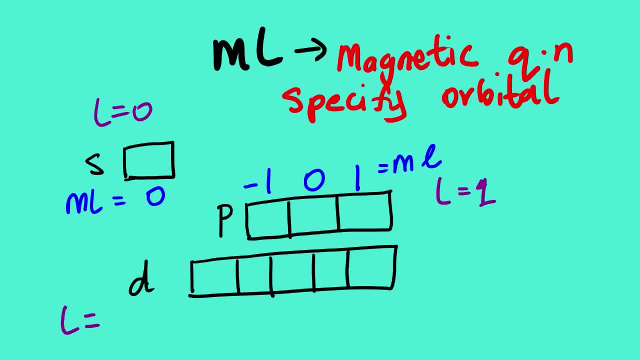 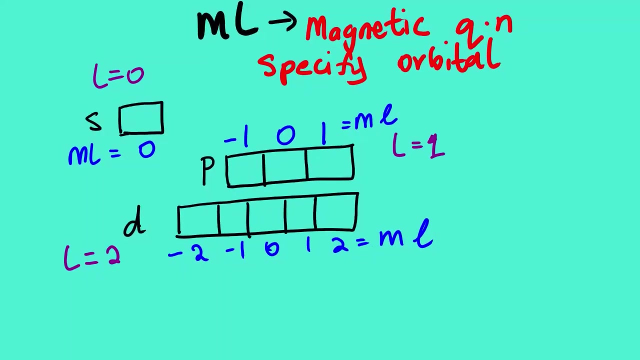 the d orbital has the sub-level 2.. So this simply means that the first orbital it will be negative 2, negative 1, 0, 1, 2.. That is the magnetic quantum number. Now looking at the f orbital, 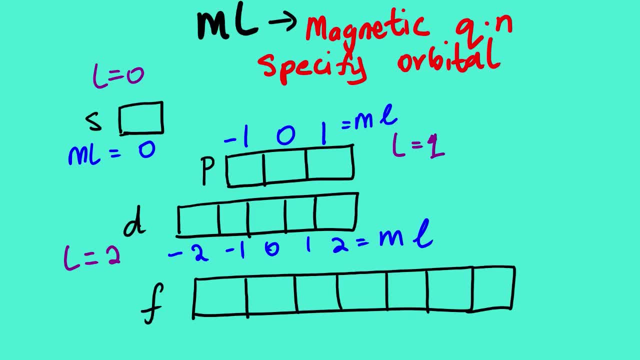 it has 7 orbitals, Then you should know that l is equal to 3.. Then it simply means that we are going to start our magnetic quantum from negative 3, negative 2, negative 1, 0, 1, 2, 3.. 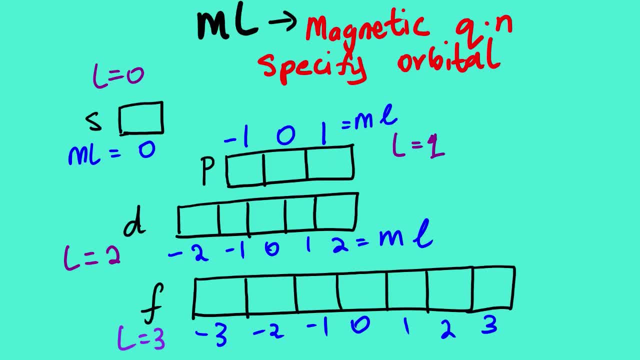 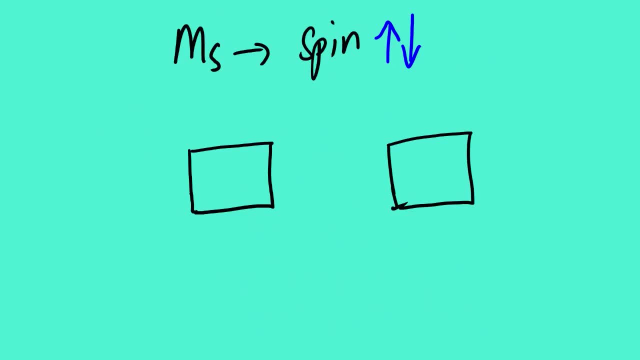 So this is what you need to know about quantum. I mean magnetic quantum number. Our last quantum number is ms, which is the electron spin. Now we know that from the orbital diagram, or the orbital energy level we have, actually from the orbital diagram. 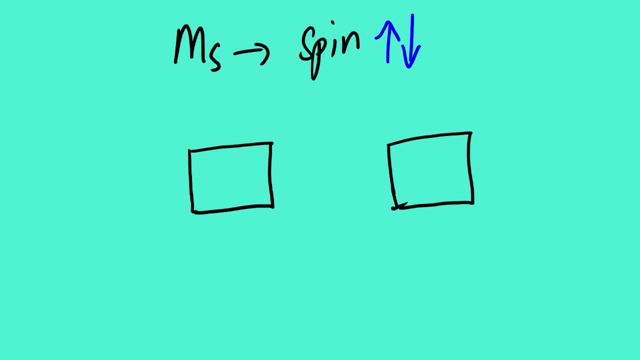 we have boxes and electrons inside the boxes. Now if the electron it faces up, it means the video of ms will be positive 1 over 2.. Then if it faces down, it means our ms will be negative 1 over 2.. 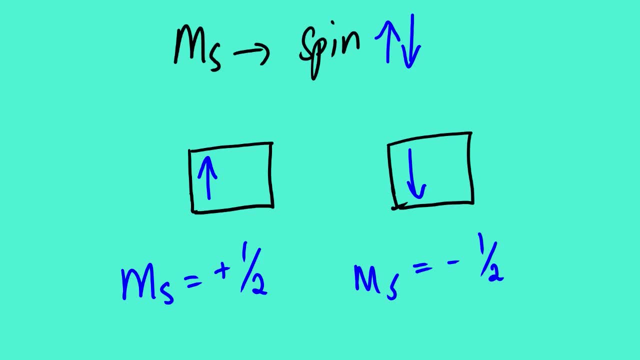 So that's what you need to know about the electron spin. It's either 1 over 2 or negative 1 over 2.. Now let us look at examples. Suppose we are given this electron as our equation and then we want to know: 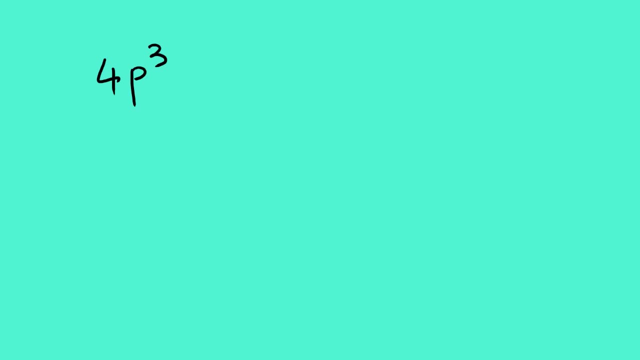 the four quantum numbers of these electrons, The value of n, the principal quantum number. It's simple, because what you see here, this is the energy level. So it simply means n is equal to 4.. Then we go to our sub-level. 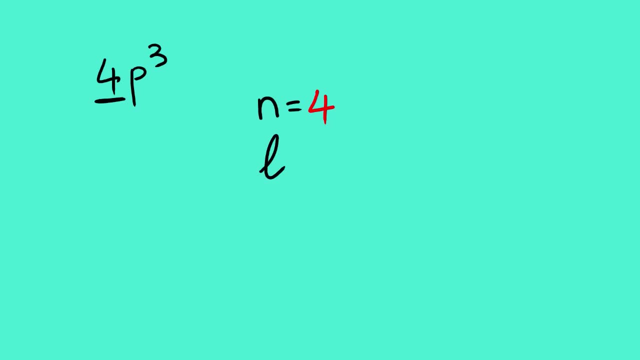 or angular momentum quantum number. We actually know that for s, l is equal to 0, for p, l is equal to 1.. So the answer to this: it's equals to 1.. And then we are left with m. 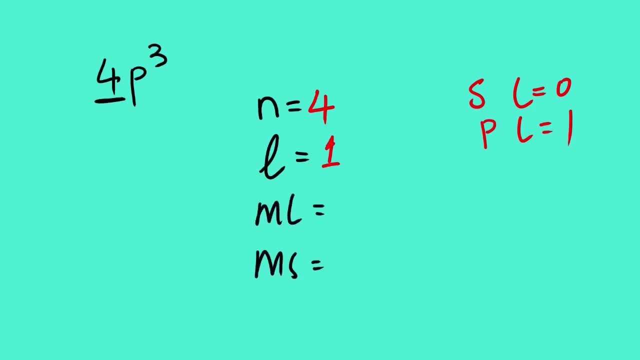 l and ms. How do we determine m? l? We are dealing with p orbital. We know that we have three boxes under p orbital. And then, what is important, You should know that p1, it means we are looking at p orbital. 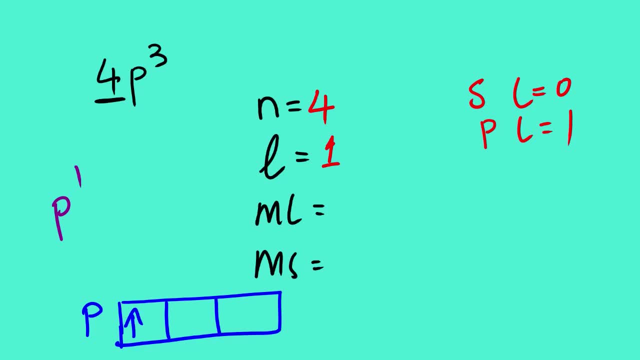 and then we only have one electron. For p2, we are going to have two electrons under p orbitals. So for p3, it means we are going to have something like this for p3.. So in this case, remember m l under p orbital. 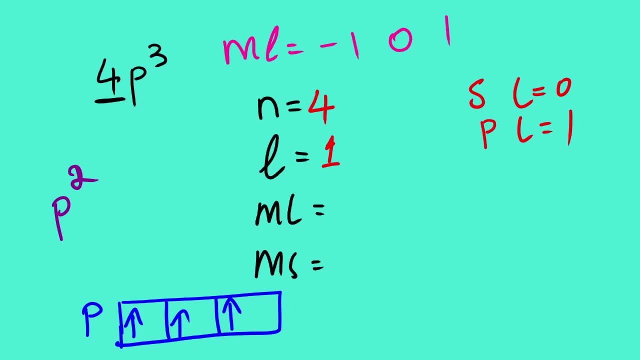 can be negative 1, 0, 1.. So we look at the last electron. Where is it? So this is negative 1, 0, 1.. So the last electron is on the last orbital, which is 1.. 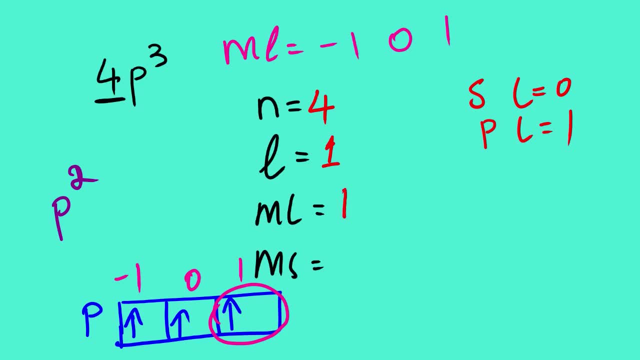 So m l is equals to 1.. And then ms is the electron facing up or down? It's facing up, So ms is equals to 1 over 2.. So these are the four quantum numbers for this specific electron. Let us look at another example. 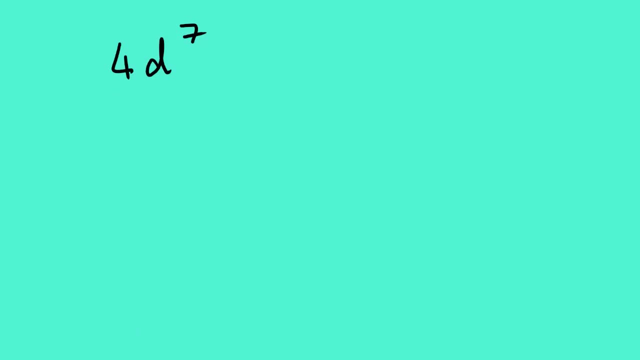 So, looking at 4d7, it's another electron- We need to find the four quantum numbers, So the value of n. we know that it's in the fourth energy level, So it's four. And then we look at l. 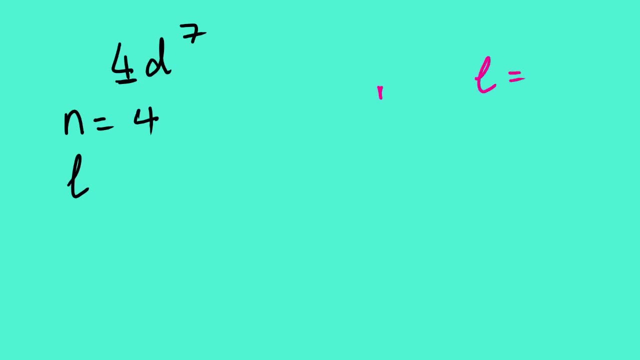 A quick reminder: we know that l for n is equals to 1.. l is 0.. n is equals to 2.. l is equals to 1.. n is equals to 3.. l is equals to 2.. n is equals to 4.. 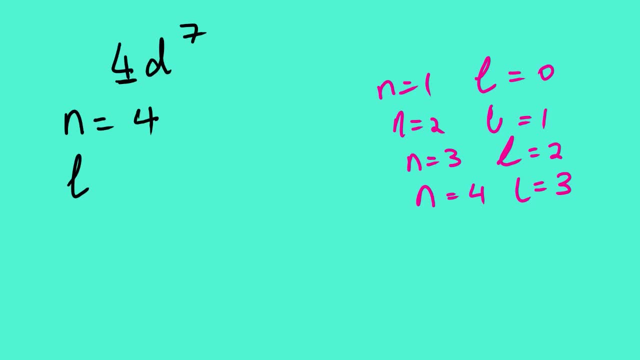 l is equals to 3.. Another reminder we should take note: remember that for this it's s, For this it's p, For this it's d, For this it's f. So this simply means that for 4d7,. 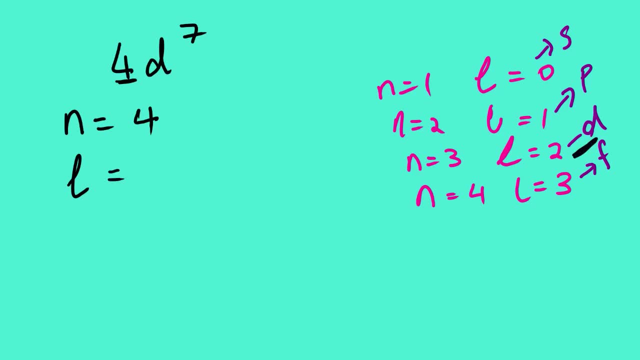 our l is equals to 2.. And then for ml, we need to draw the orbital diagram of d. So it will have five boxes: One, two, three, four, five, Okay, And then we know that it will start from negative 2,. 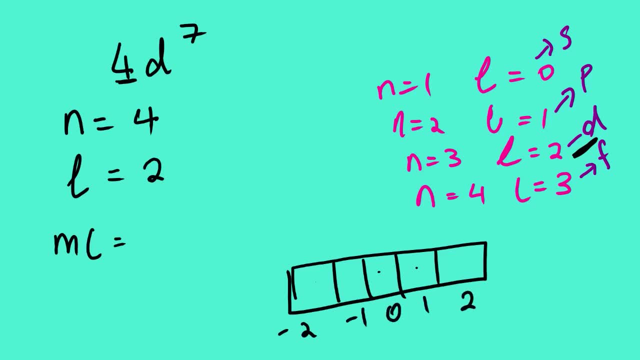 negative: 1, 0,, 1, 2.. Now, remember we are looking for seven electrons, So it will be 1,, 2, 3, 4,, 5, 6, 7.. So you can see that the seventh electron is on negative 1.. 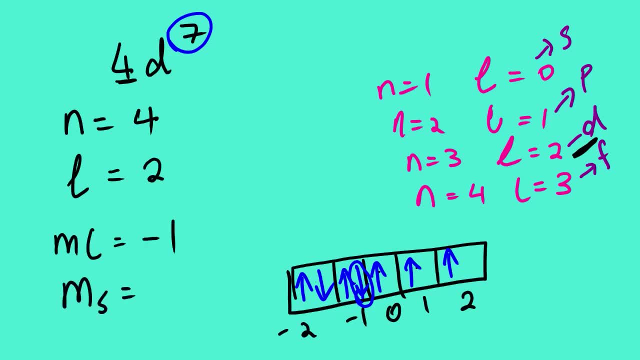 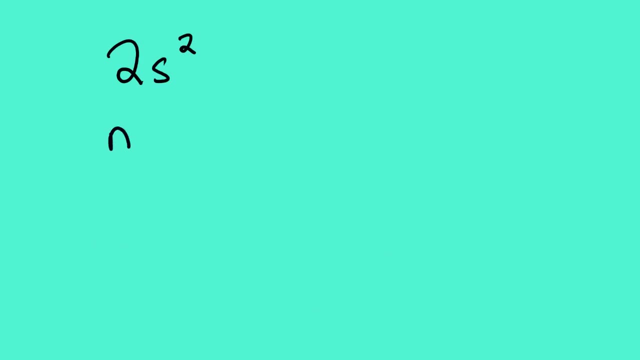 So the ml is negative 1. For ms, since the seventh electron faces down, so it will be negative 1 over 2.. Let us look at another example. What about 2s2?? So the value of n is on the second level. 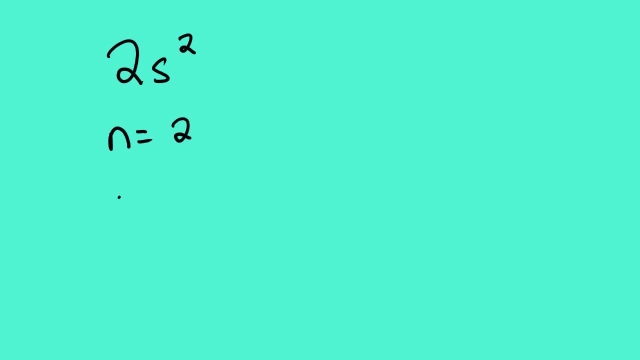 It's 2.. The value of l- since we are dealing with s orbital- is 0. Then we're looking for ml and ms. Now we know that s has only one orbital, So there's no choice. It means ml will be 0.. 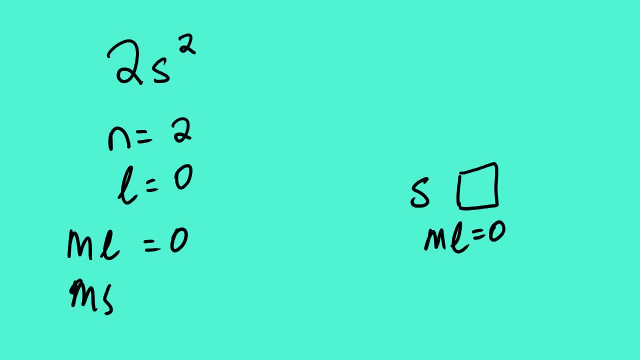 And then for ms let us fill in two electrons, So it's 1, 2.. Since the second electron faces down, this simply means the ms will be negative, 1 over 2.. Let us look at another example: 1s1.. 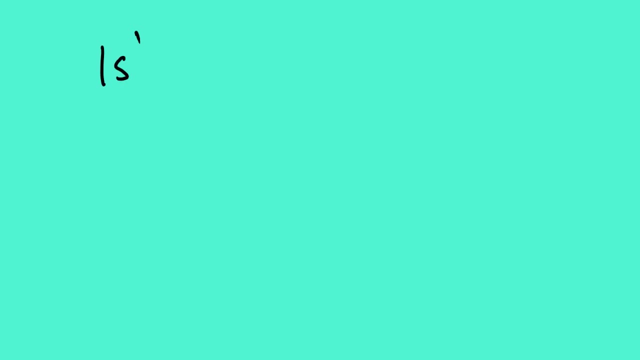 Let us find the four quantum numbers for this electron. So n is equal to 1.. l is equal to 0.. Since we're dealing with s orbital ml, and ms You know that s only has one orbital, So ml is the same as the previous example.